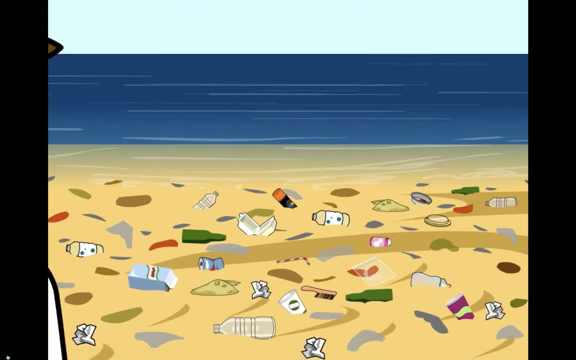 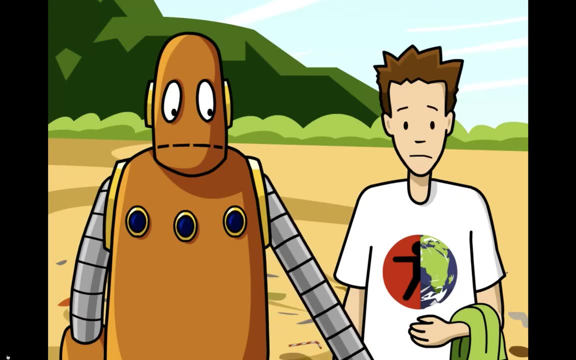 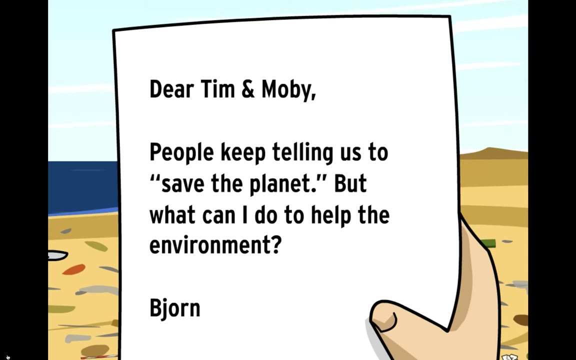 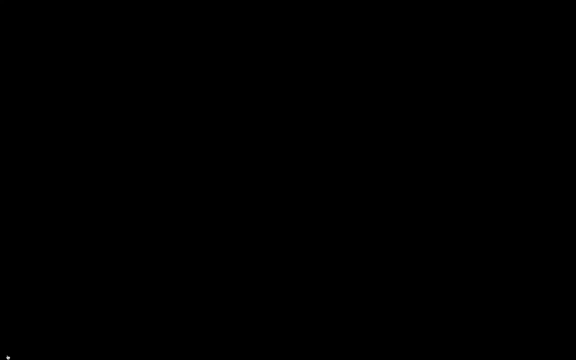 Look at all this trash, Moby, Dear Tim and Moby. people keep telling us to save the planet, but what can I do to help the environment From Bjorn? That is a great question. Three of the best ways I can think of are conserving, cleaning up and chiming in. 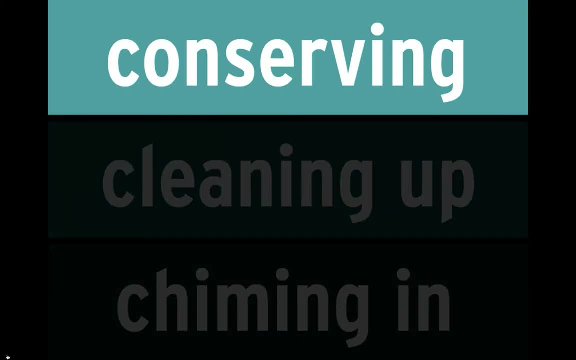 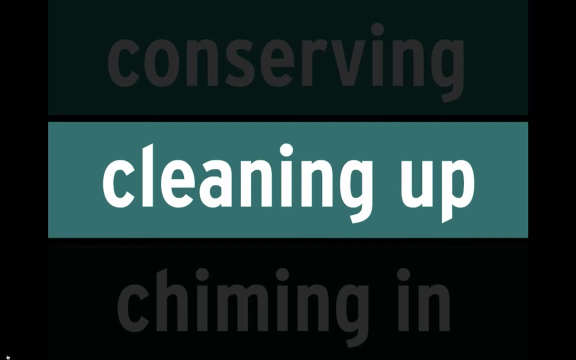 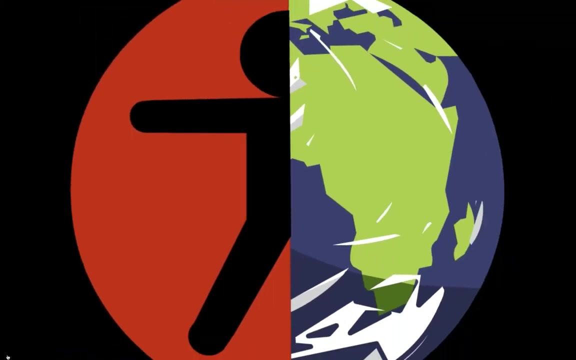 Again, conserving means using less of things like energy and manufactured goods. Cleaning up means cleaning up after yourself, for sure, but also after others, when you can't. And chiming in that means you should speak up about protecting the environment. Well, for many thousands of years, humans have been using the Earth's natural resources. 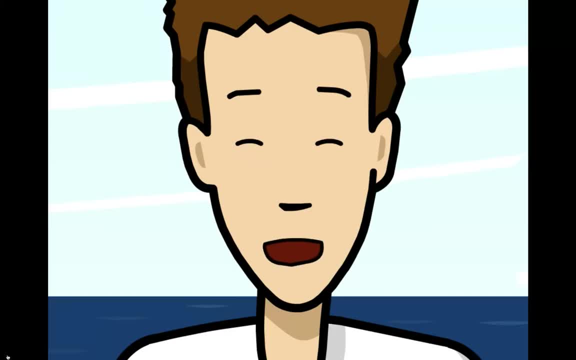 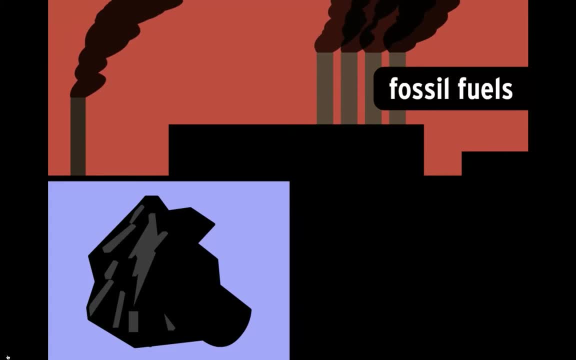 things like the air we breathe and the water we drink. But we've only made a major impact on the environment over the last 200 years or so. For example, we began. We began burning fossil fuels like coal and petroleum during the Industrial Revolution of the 18th and 19th centuries. 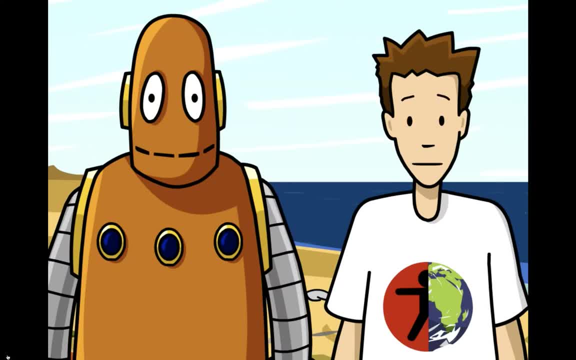 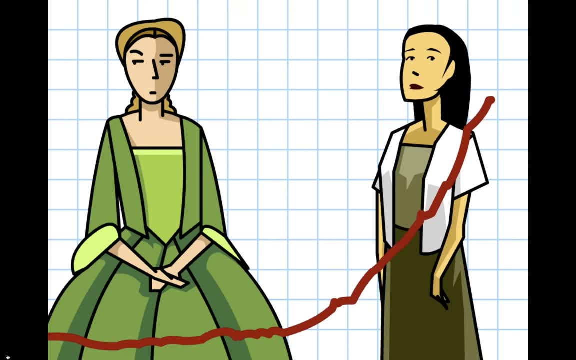 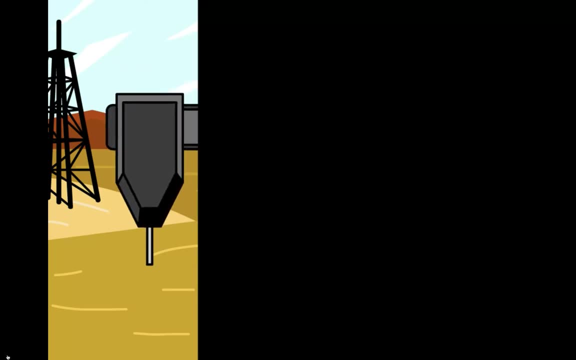 Not only was this the beginning of pollution as we know it, it also marked the start of a huge population boom. Between 1800 and the present, the world population shot up from 1 billion to 7.7 billion. The more people there are on the planet, the more natural resources we use, the more chemicals we release and the more waste we produce. 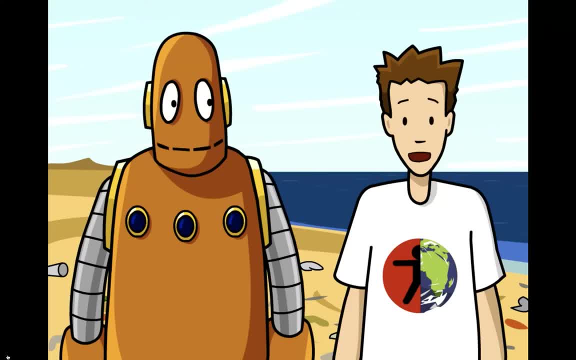 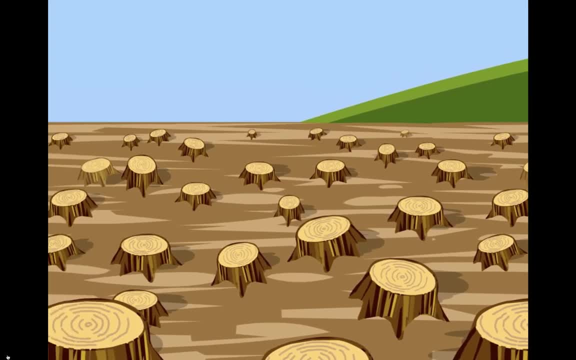 Well, there are lots of reasons why this is bad for the planet and us. For instance, whole forests have been cut down in order to produce wood for homes, furniture and paper. Destroying forests also destroys the homes of animals and other wildlife, which can cause organisms to go extinct. 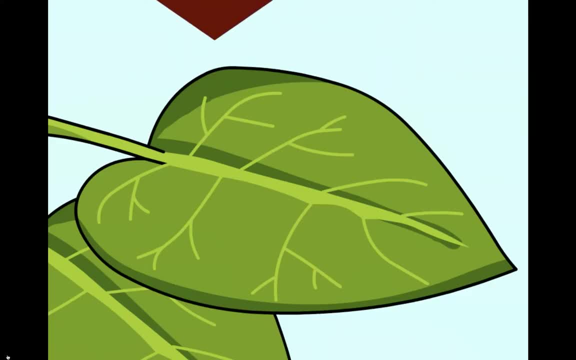 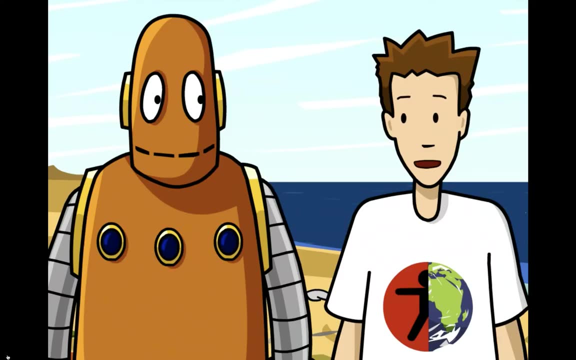 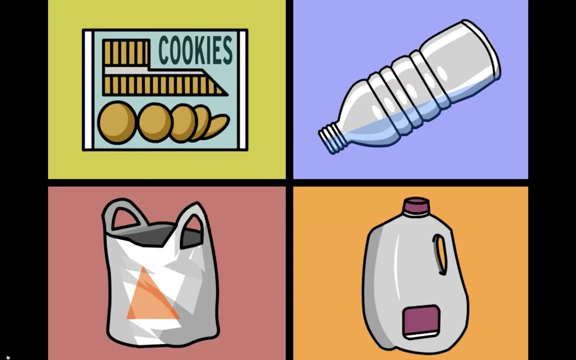 And trees themselves are important to our health. Plants get rid of carbon dioxide and produce the oxygen we breathe, so we need to have them around. Yeah, lots of the stuff we We buy every day messes up the planet too. Take the plastic containers that so many things come in. It takes a lot of oil to make just a little plastic. 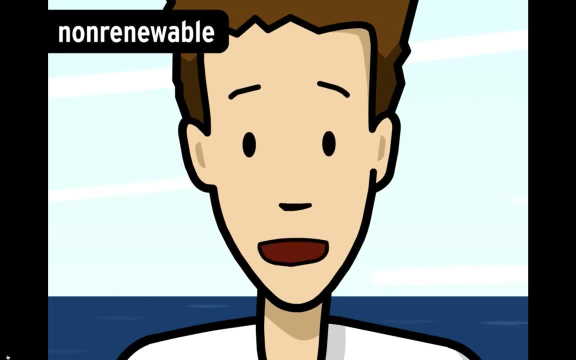 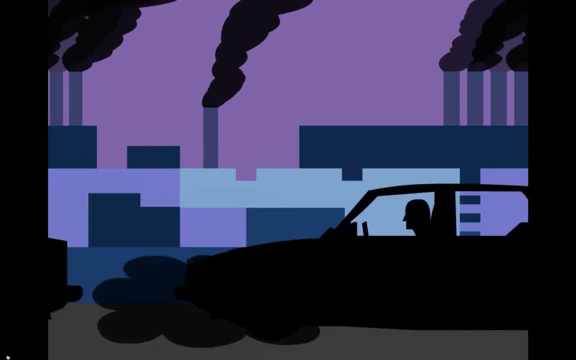 Oil and other fossil fuels are non-renewable sources of energy. There's only so much on the planet. Plus, when these fuels are burned, carbon dioxide, nitrous oxide and methane are produced. These pollutants don't just damage our atmosphere and our lungs, they also contribute to global warming.